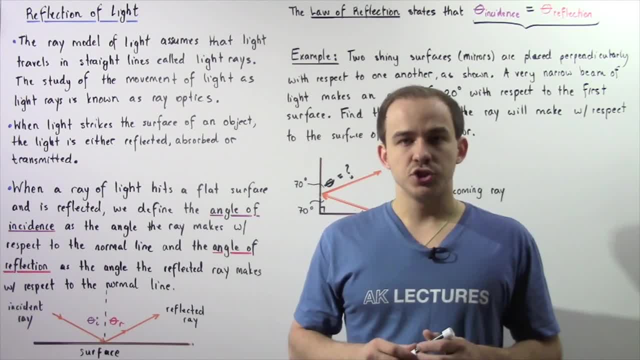 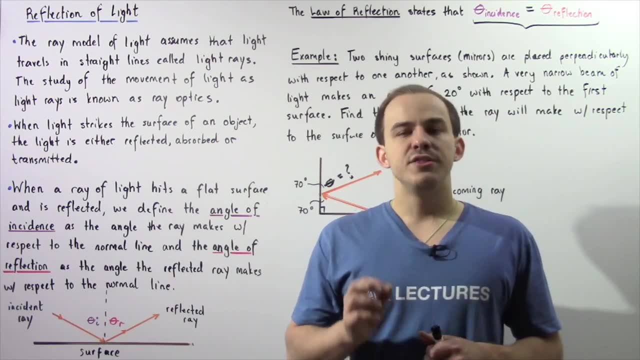 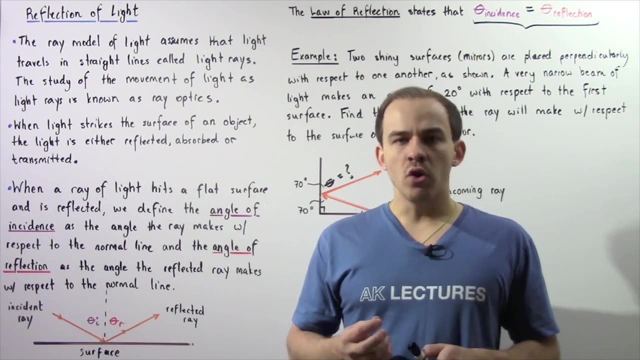 In our discussion on electromagnetic radiation, we basically said that visible light is one form of electromagnetic radiation that has a specific range of values for the frequency and the wavelength. Now, in order to study the properties, the behavior and movement of visible light, 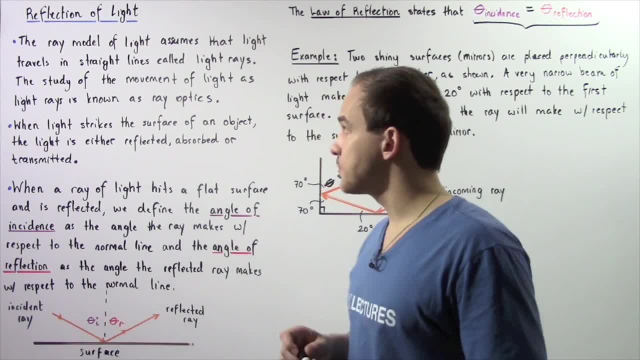 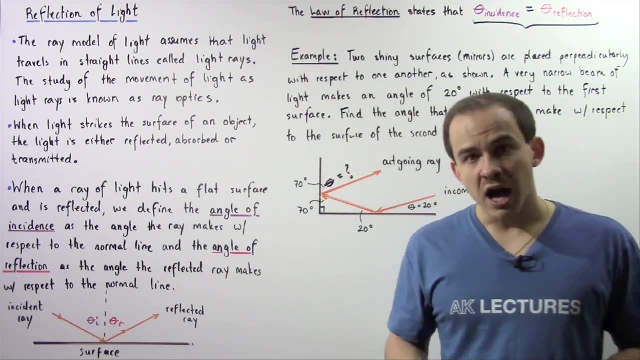 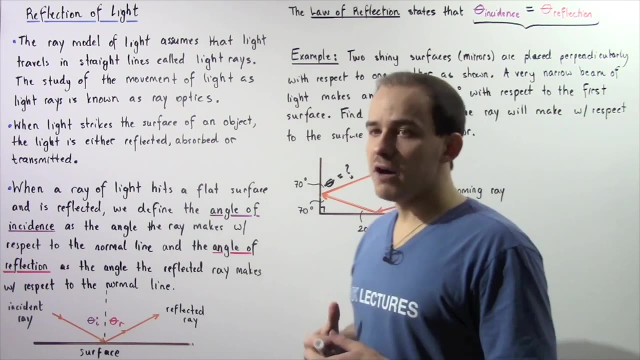 we have to make certain assumptions about light. So the ray model of visible light assumes that light travels in straight lines, in straight pathways, known as light rays. Now the study of movement of light in the form of light rays is known as ray optics. 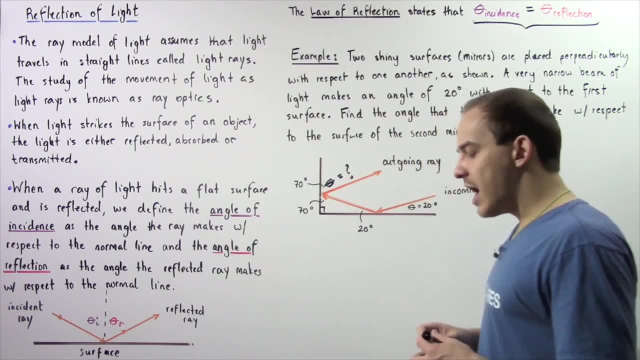 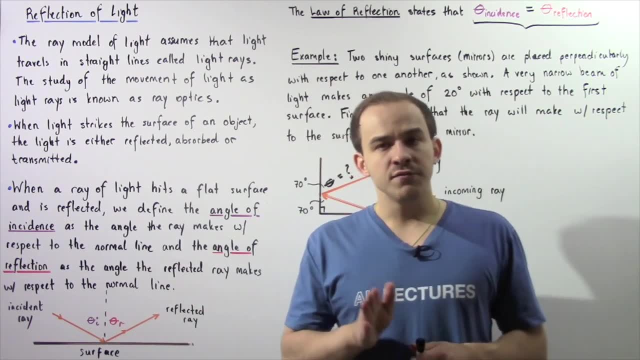 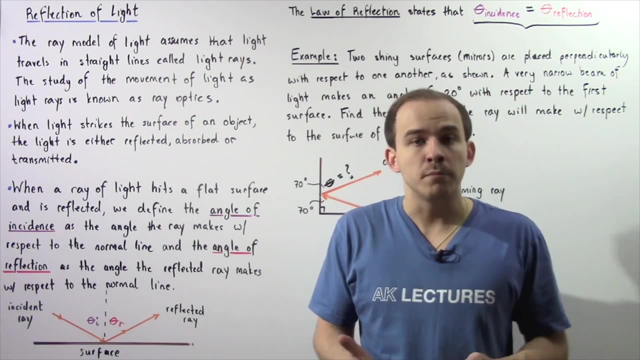 or simply geometric optics. Now, whenever visible light, or simply light, travels in straight lines, we have to make certain assumptions about light. So the light that strikes the surface of an object, one of three things can take place. The light can either reflect off of that surface. it can be absorbed by the molecules inside that. 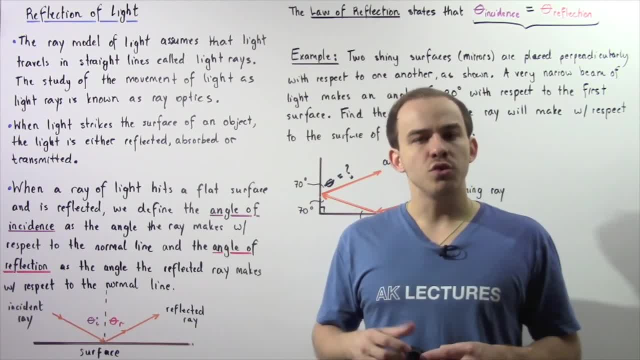 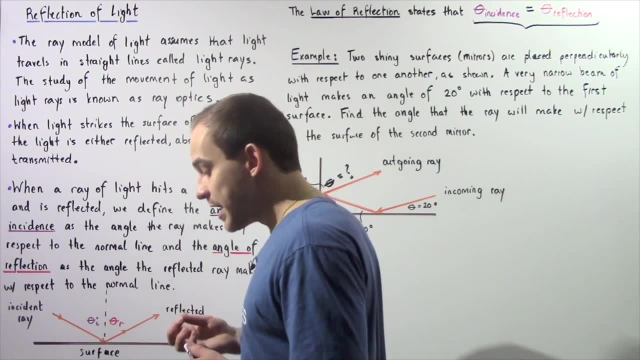 surface or the light can be transmitted through that surface. So let's suppose light is traveling and it hits the surface of glass. So because glass is essentially transparent, some of that light will be reflected and some of that light will be transmitted. So let's suppose 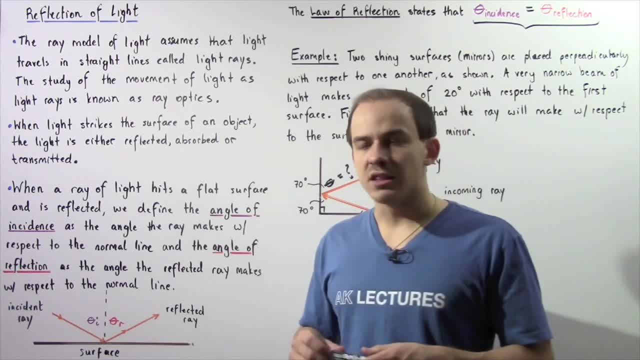 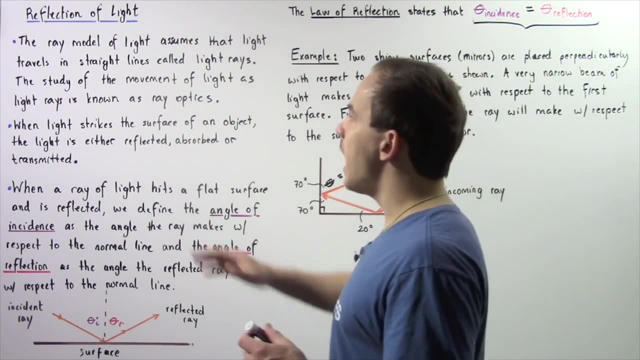 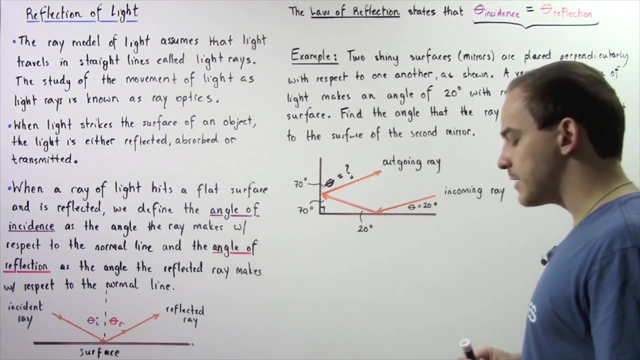 light is reflected, some of that light will be absorbed and some of that light will be transmitted through glass. Now in this lecture we're going to focus primarily on the reflection of light off of surfaces and we're going to look at the law of reflection. So when a ray of visible 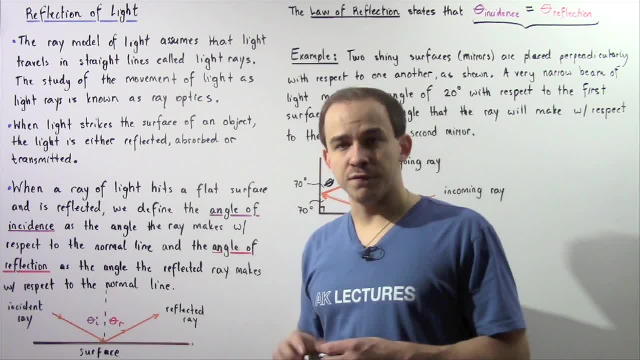 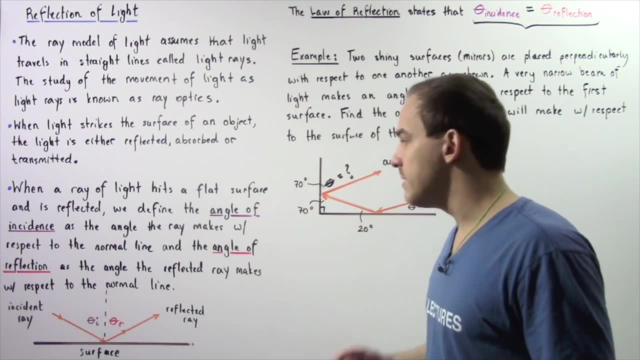 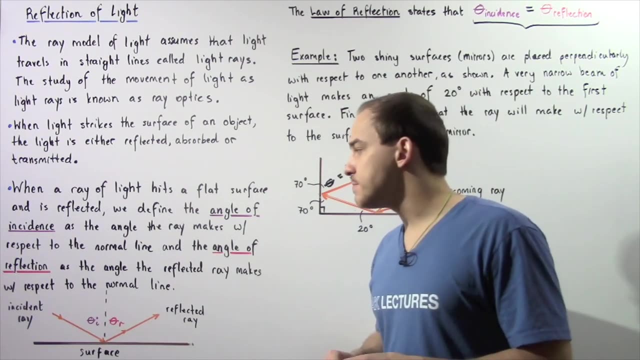 light hits a flat, shiny surface and is reflected. we define the angle of incidence as the angle of reflection that the incoming or incident ray makes with respect to the normal line that is perpendicular with respect to the surface, And we define the angle of reflection as the angle that 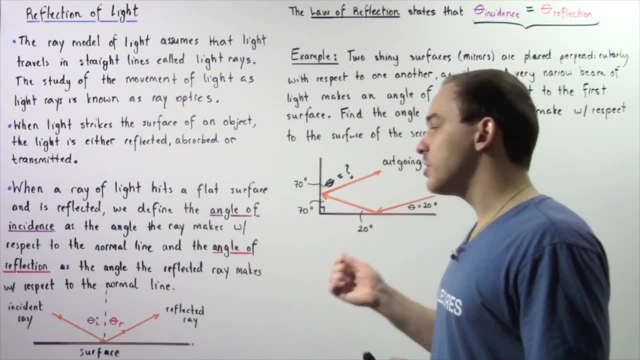 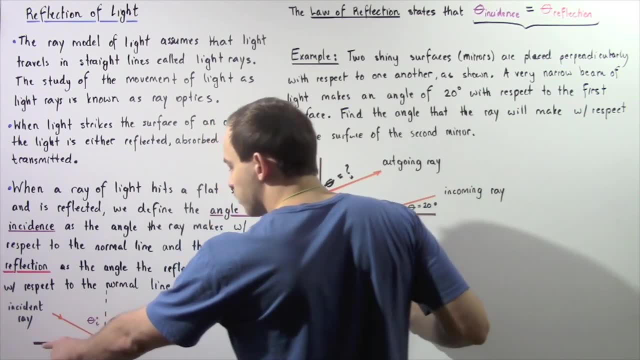 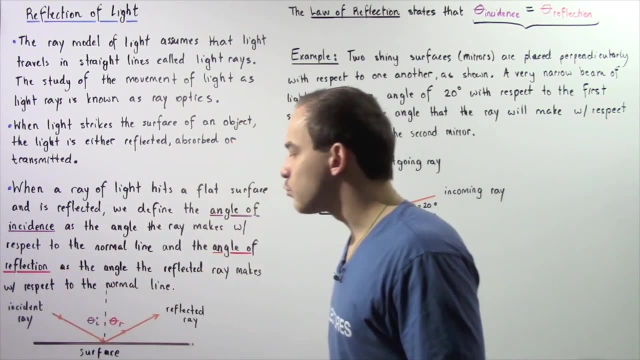 the outgoing or reflected ray makes with respect to the normal line. So let's examine the following diagram. Let's suppose this brown region is our shiny surface And this is our incoming light ray, also known as the incident ray. So the incident ray will travel. 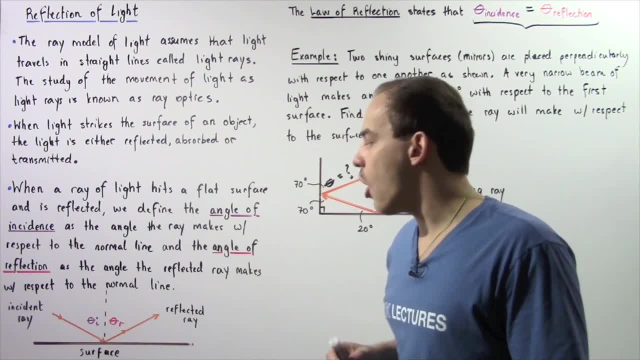 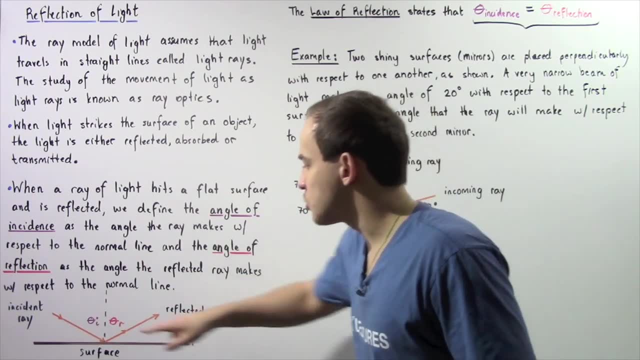 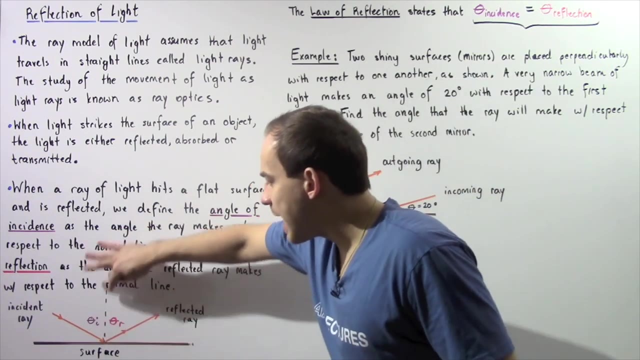 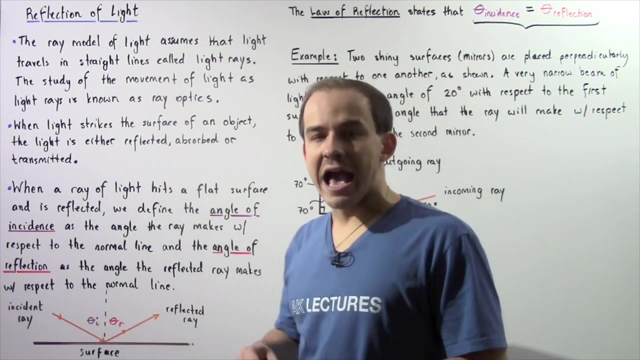 will eventually hit the surface and will reflect off of that surface, And this reflected ray is shown as the following arrow. So we have the orange arrow coming in and the orange arrow coming out. Now this dashed line represents our normal line. It's the line that is perpendicular to the surface of our object, So this angle is known as the angle. 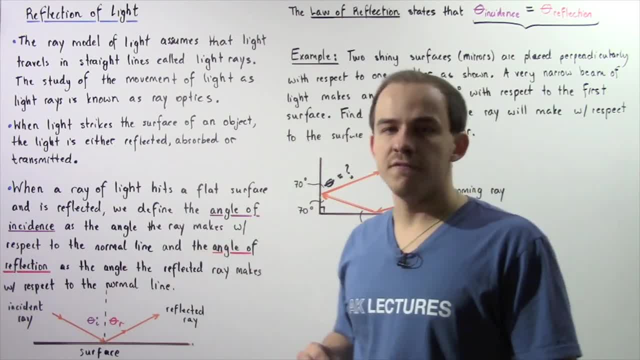 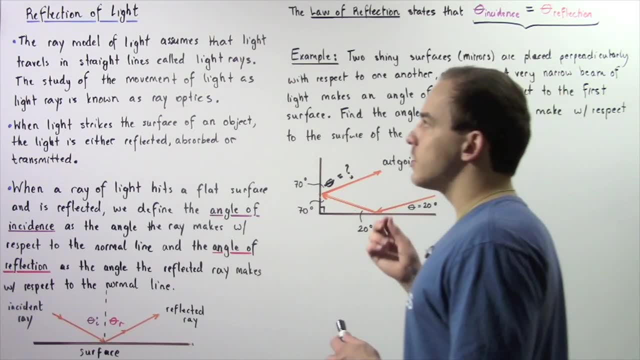 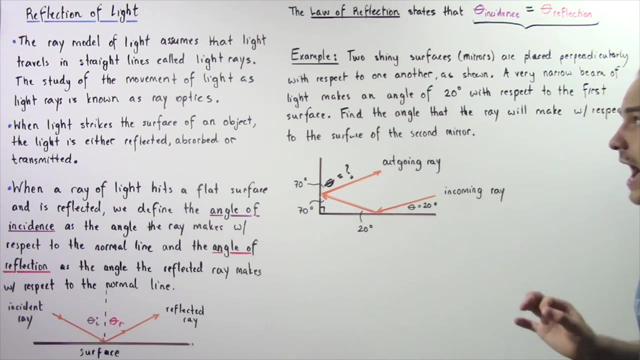 of incidence, and this angle is known as the angle of reflection or the reflected angle. Now let's discuss a law known as the law of reflection. So the law of reflection essentially states that any time light reflects off of a flat surface, it's the angle of incidence that is known as the angle of. 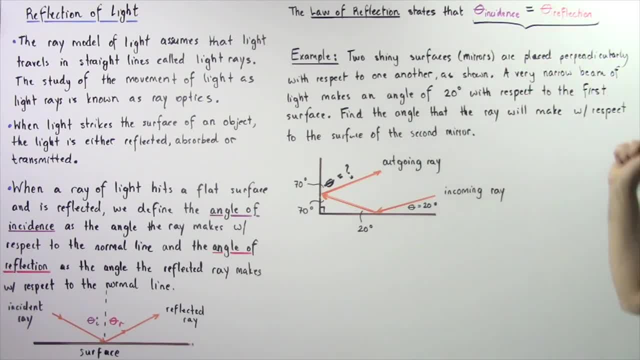 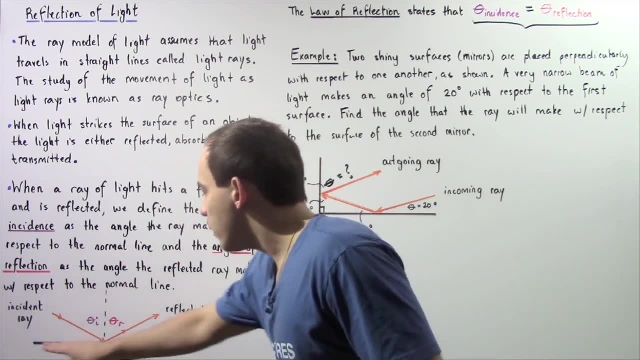 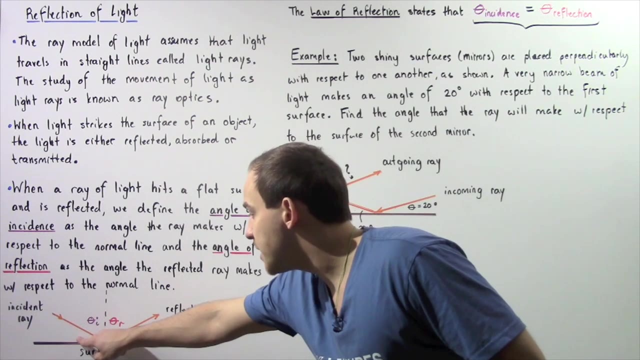 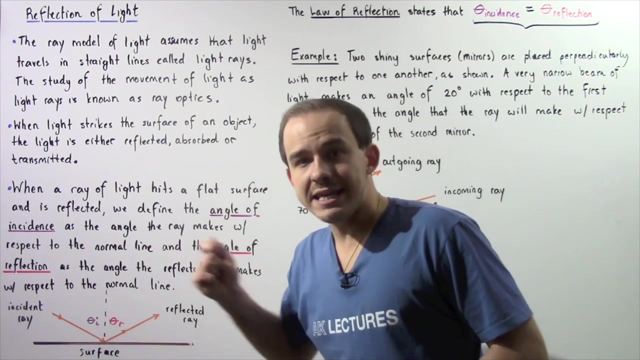 incidence. So the angle of incidence will equal to the angle of reflection. So these two angles will be equal. Now, if we assume this is a flat surface and these two angles are equal, that basically implies that this angle is also equal to this angle, because the sum of these angles is equal to 90 degrees. because this line is: 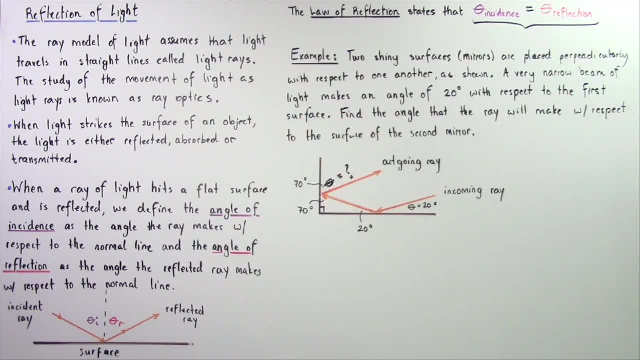 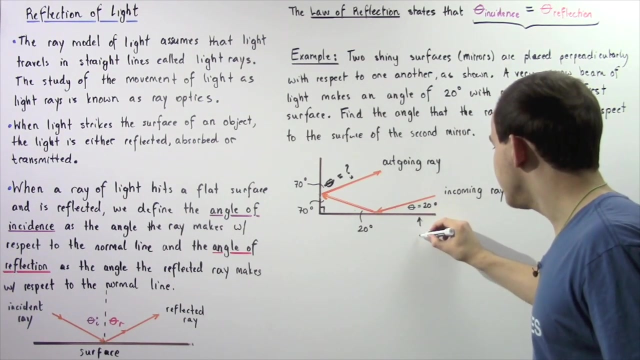 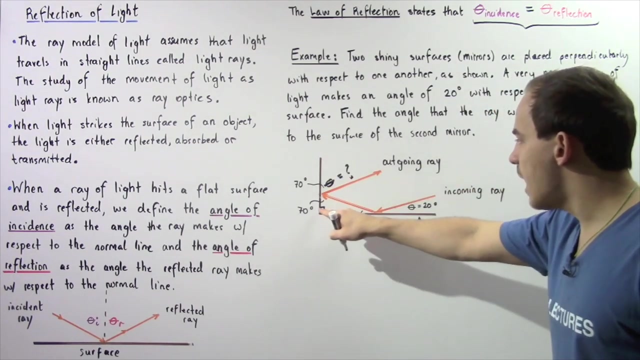 perpendicular to the surface. So let's look at the following example that will essentially apply the law of reflection. Let's suppose two shiny surfaces, let's say mirrors, are placed perpendicularly with respect to one another, as shown in the following diagram. So this brown line is surface number one and this line is surface number two, And these lines are: 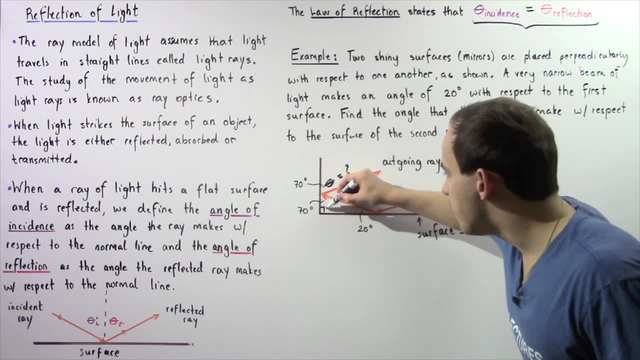 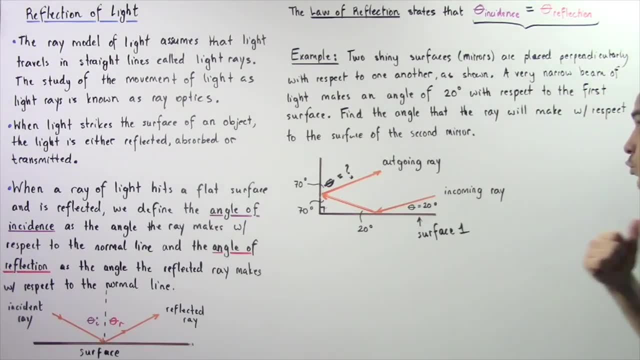 perpendicular with respect to one another, as shown by the following perpendicular symbol. Now a very narrow beam of light, a light ray, is traveling and hits surface number one with an angle of 20 degrees, as shown in the following diagram. So we want to find the angle that the light ray makes with respect to the surface.